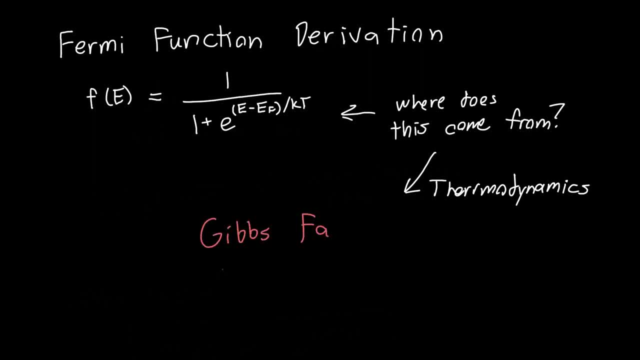 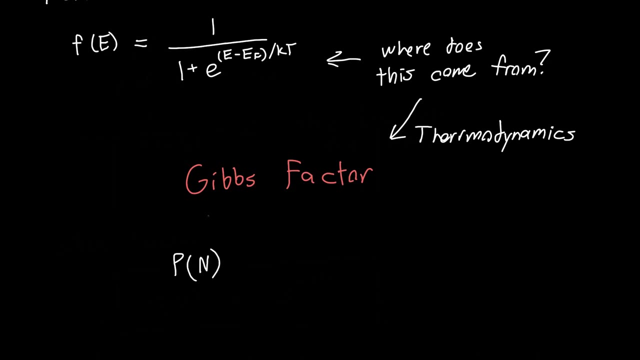 the Gibbs factor And it's got a kind of a fancy name named after this guy named Gibbs, which personally I think is a pretty cool name. And what this guy Gibbs said is that the probability of a given state being occupied with n electrons. they can be any particles, but we're just going to. 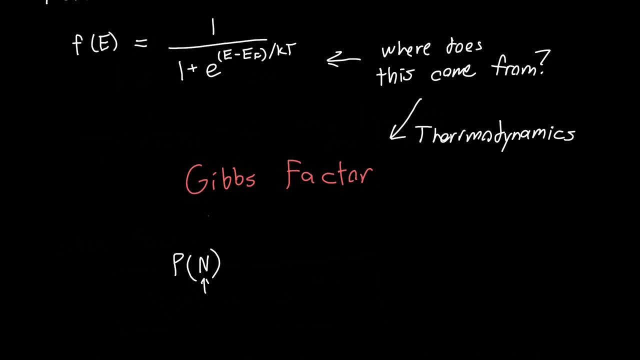 deal with electrons here is just proportional, so not equal to, but proportional to the negative exponential of the total energy of that state, with n electrons divided by kt. And this is probably the most important formula in all of thermodynamics, other than perhaps the thermodynamic identity, but we won't cover that here. 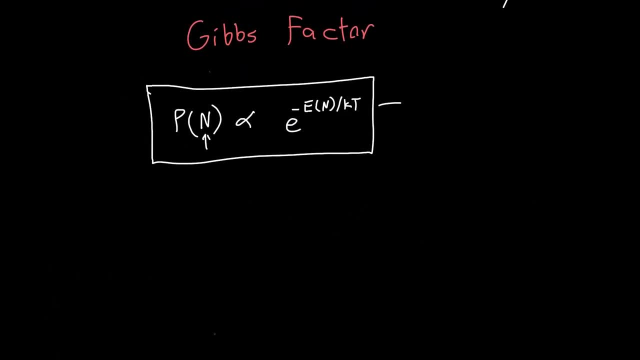 So how do we convert this probability of a given state being occupied- because this is the probability for a single state being occupied with n electrons- how do we convert this into our Fermi function? the thing that we're going to do is we're going to add in the same thing that we want. 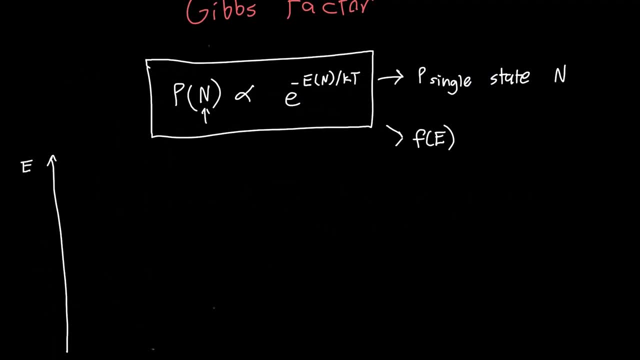 because we know, in reality we're going to have a bunch of states with a bunch of different energies. So let's say, if I've got energy on the y-axis and we've got, I don't know, five states at this energy- I don't know, maybe this is 2 eV or something- four states at this energy obviously. 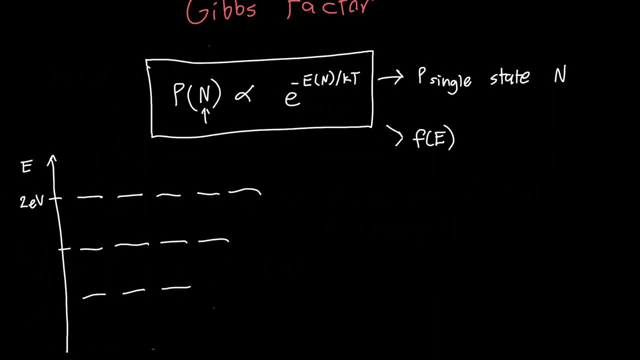 this is a hopeless underestimate, but you, it's just to illustrate a point. there's going to be different numbers of states at different energies, And this is going to be determined by the density of states, function g, which we calculated previously, And so we want to find the percentage of states that are occupied. 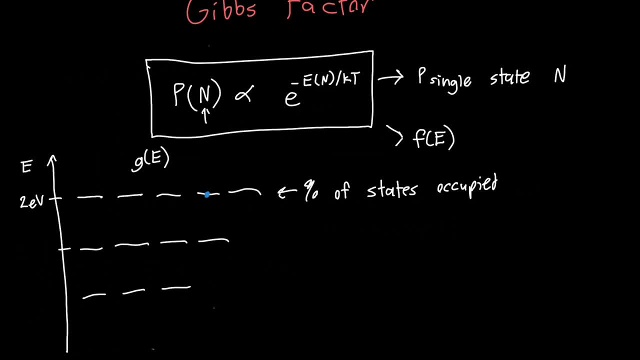 with electrons. So we want to know how many of these states have an electron inside them. And the beauty of the Gibbs factor is that if I know the probability of a single state being occupied, then that's just the same exact thing as the percentage of the states occupied If the 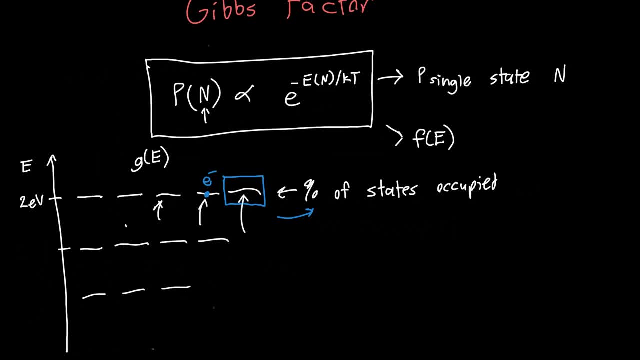 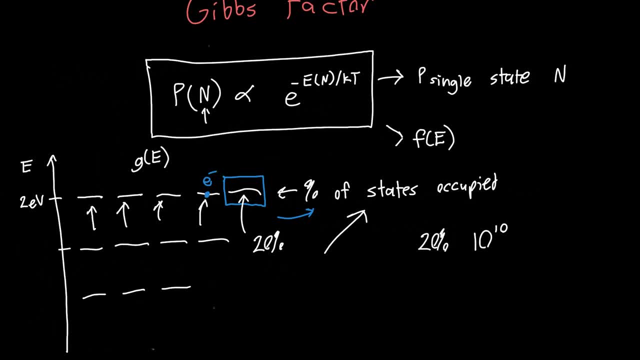 almost exactly 20% of those states being occupied. So if we can calculate the probability of an electron being occupied with an electron inside an electron, then we can calculate the of a single state being occupied. that will give us the percentage of all the states at a given. 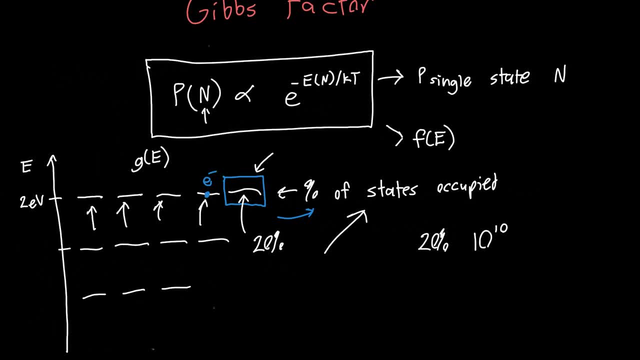 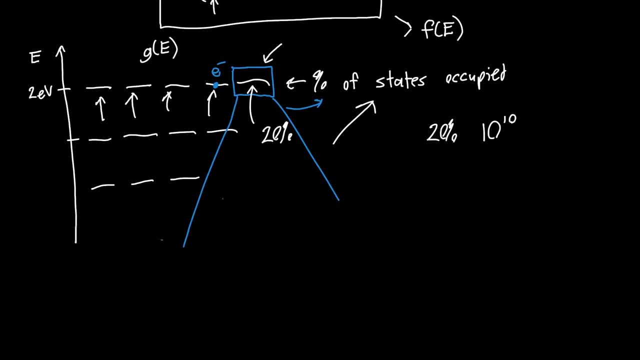 energy that are occupied. so let's zoom in on a single state, let's take a look at this, this single state, and let's draw it nice. and let's draw it nice and big. so state we know that the probability of this state having n electrons in it is proportional to e, to the minus energy. 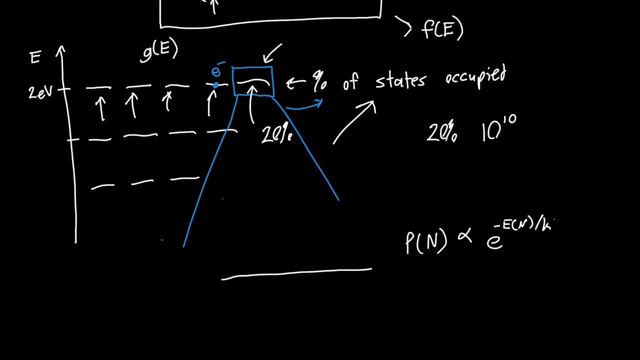 of that state with n electrons divided by kt. but we know from the Pauli exclusion principle that there's either zero electrons. so there's either zero electrons, in which case the state is unoccupied, so the state is just a blank state, or there's one electron, in which case the state has an electron in it. so 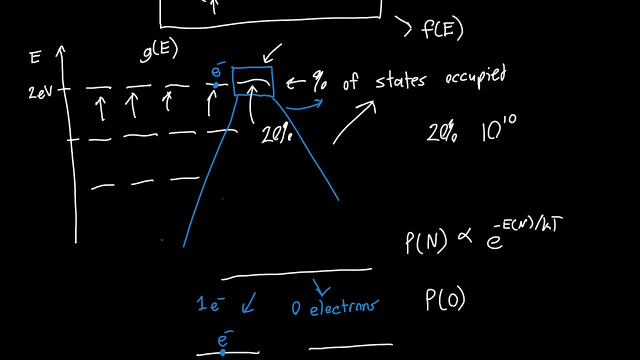 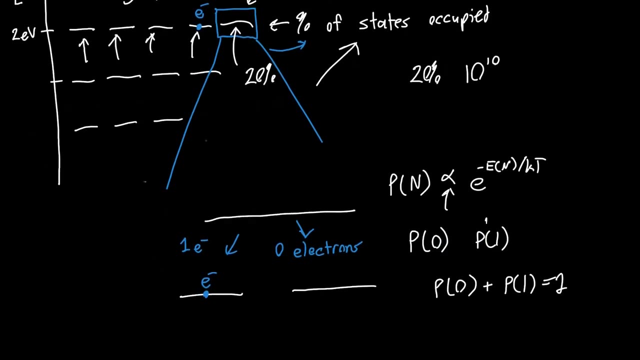 there's only two possible cases here, p of zero and p of one, and from the definition of probability we know that these two have to add up to one. so p of zero plus p of one must just be equal to one, and so we can use this fact to change this alpha from an alpha to an equal sign. we can rewrite p of. 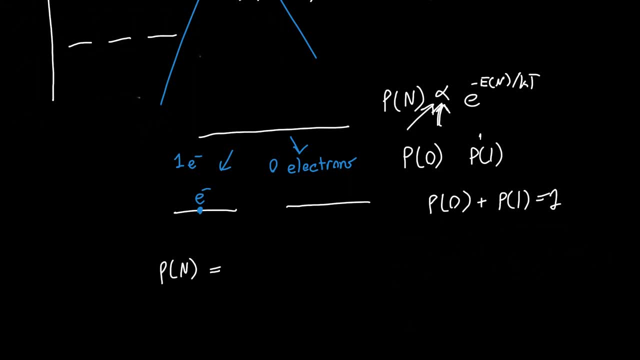 n as some constant of proportionality, let's, let's look at this again. let's call it one over z, and that's just to be consistent with the the rest of the literature on this times e to the minus energy over kt. so instead of writing proportionality, we're. 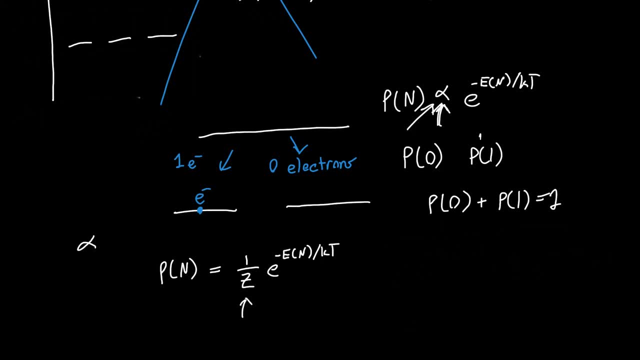 just replacing. we're saying that proportionality constant is just one over z, so okay, we can then write. we can then solve for that proportionality constant, so one over z times e to the minus, e with zero electrons divided by kt, plus one over z times e to the minus. 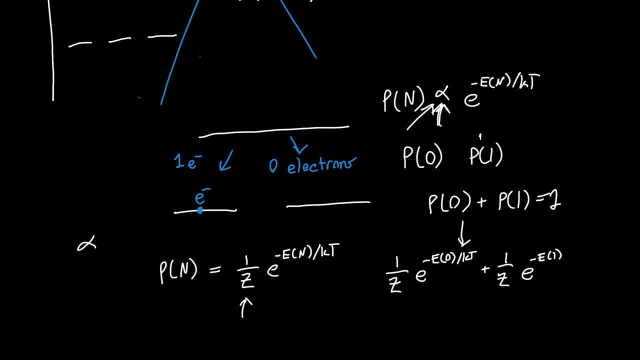 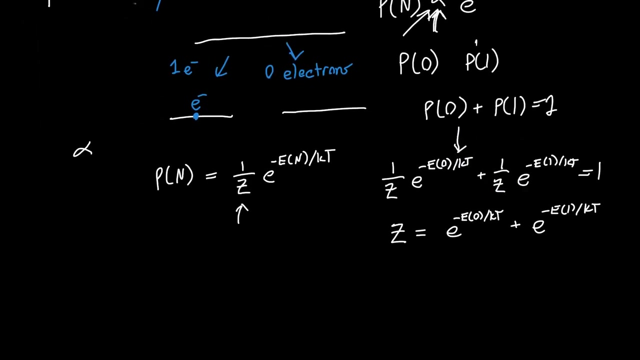 e of one electron or the energy of one electron occupying that state divided by kt is equal to one, or z um is just equal to e to the minus e, zero over kt mine, or plus e to the minus e, one over kt. and we're almost finished. we said that our fermi function was just the same thing. 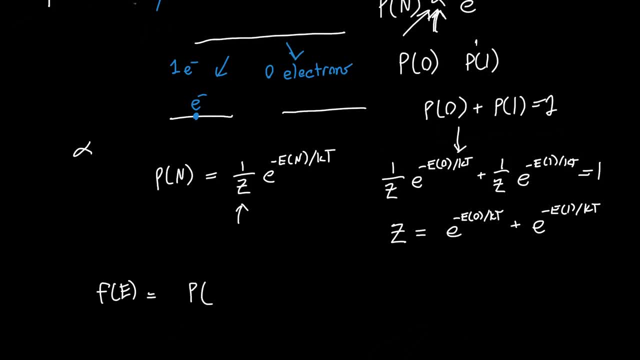 as the probability of the state having one electron. so we know the proportionality constant now, so we can just directly write that we know that it's one over z times the or, not, sorry, not e- times the exponential, the negative exponential of the energy of that state. 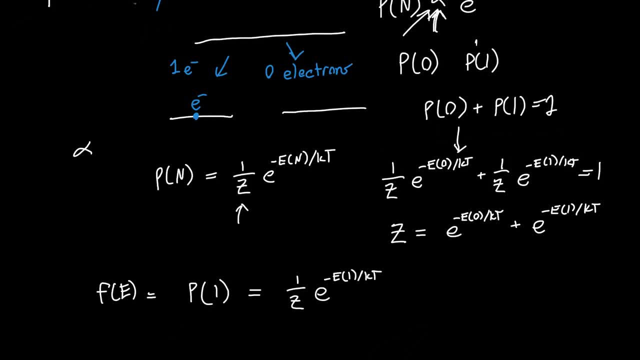 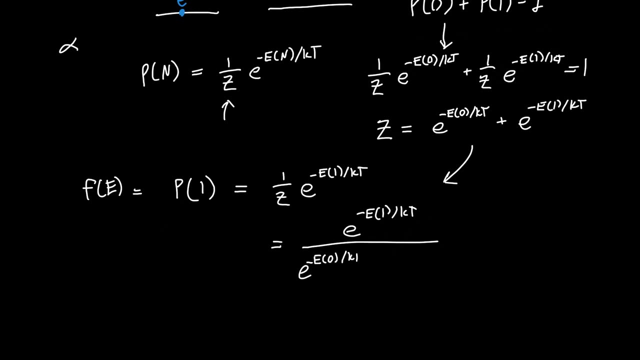 with one electron divided by kt. so we know what z is. we can just plug it in. so that's just e to the minus e1 over kt divided by uh, e to the minus e zero over kt, plus e to the minus e1 over kt, and we can make this a. 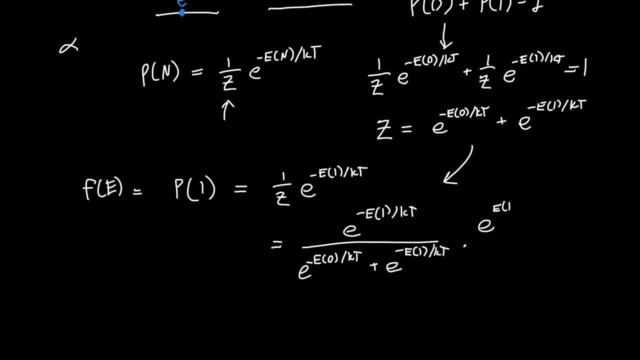 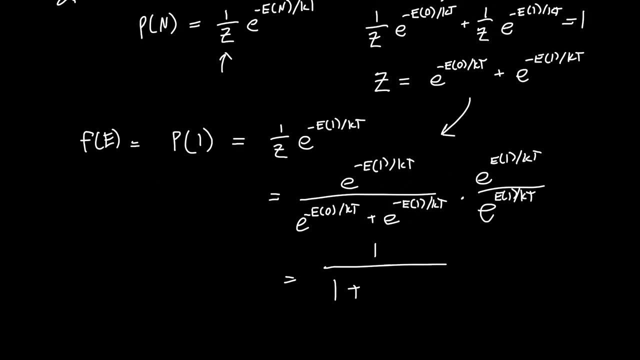 little less ugly just by multiplying by e to the e1 over kt, over e to the e1 over kt, simply by making just zero answers. so you can just we're gonna tell you the equation, so we can, we can take that out and replace that with this one, and then what we're gonna play. 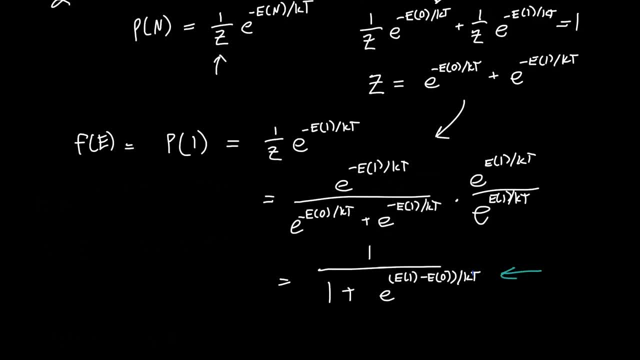 out. this is just a common trick: multiplication by one just to make it look prettier, and then our equation just becomes one: over was1, over e, to the e1to minusقط. we're so close. this function looks so much out. what is this e of n? um? so when i wrote down this e of n, what i meant to say is the kinetic. 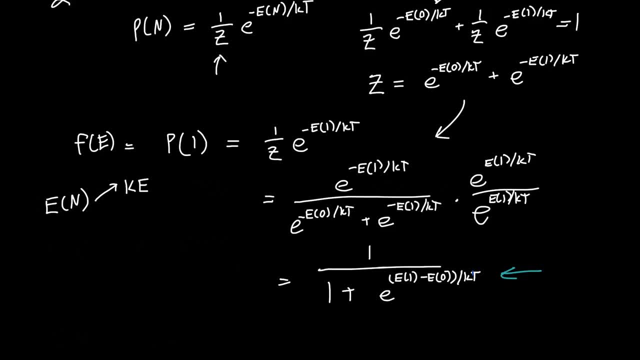 energy, so the kinetic energy of the electrons here, or the total kinetic energy of all the electrons. so since we know that the total energy uh, and so i really should have written this as k, not e, uh, to be to be less confusing. so i'll rewrite that in in the expression: 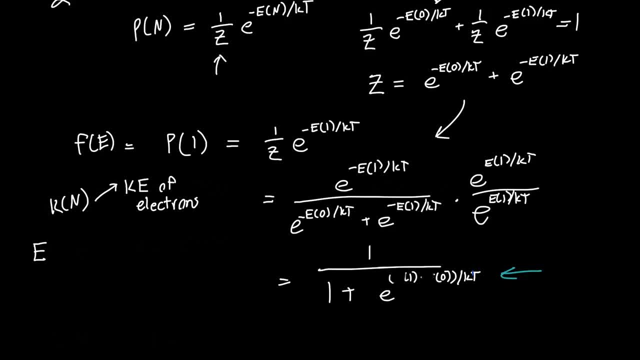 uh, so kinetic energy, kinetic energy, so the we know that the total energy is just the kinetic energy plus the potential energy, or the kinetic energy is just equal to the total energy minus the potential energy? well, for us, we actually know the total energy of these electrons: it's just the 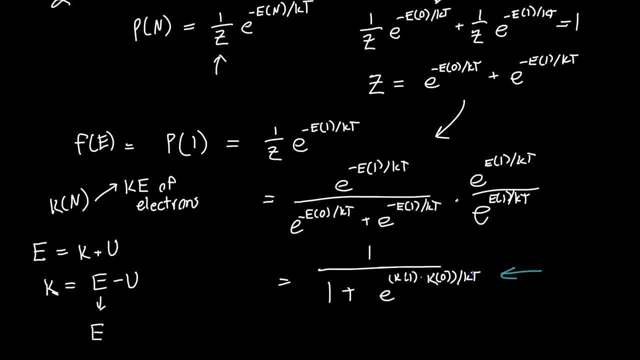 total energy of the state. uh, so i don't know es actually. let me write this as e total, because we only care about the energy of the state. so it's the energy of the state multiplied by the number of electrons in that state, minus the potential energy, which is just this thing called the chemical potential energy or, in our case, the 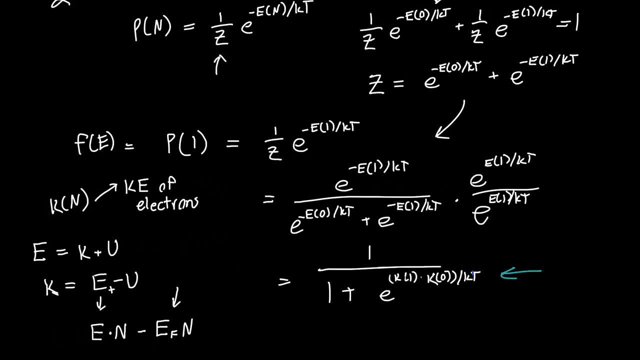 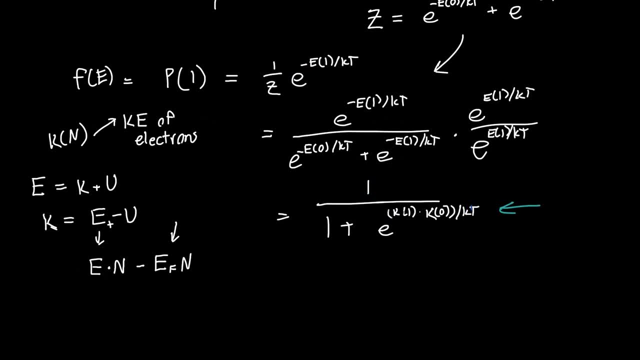 fermi potential energy multiplied by the number of electrons. and so if we evaluate the kinetic energy with zero electrons, well that's just e times the energy of the state, times zero, minus ef times zero, that's just zero. so we can actually delete this term in our uh, in our exponential over here. um what? 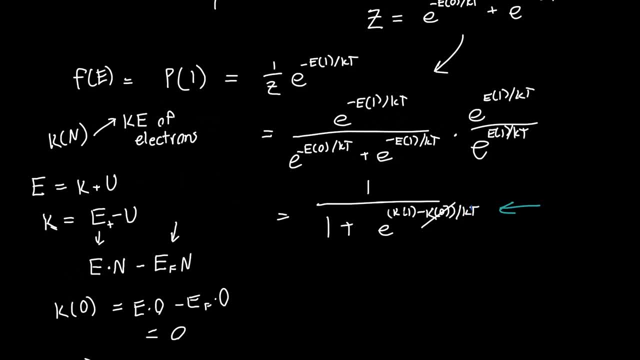 about k of one. well, that's just. we plug in: n equals one, and that's the energy of the state times one minus the fermi energy times one. and so we can just rewrite then our fermi function in its final form: one plus e to the k1, which is just e minus ef over kt, and we're done. that is the fermi function as a function of. 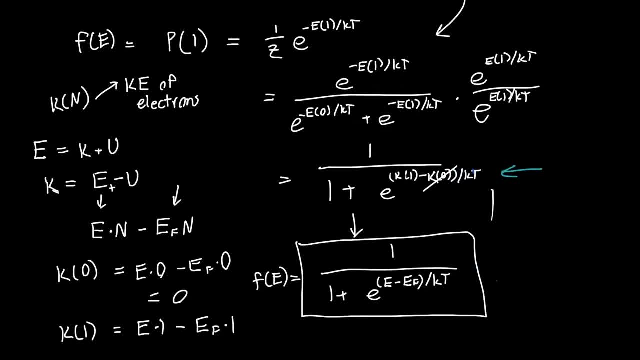 energy. oh and so i hope you enjoyed this video. if you did, please like and subscribe. uh, if you have any comments, please feel free to post them down below, and i'll see you next time.